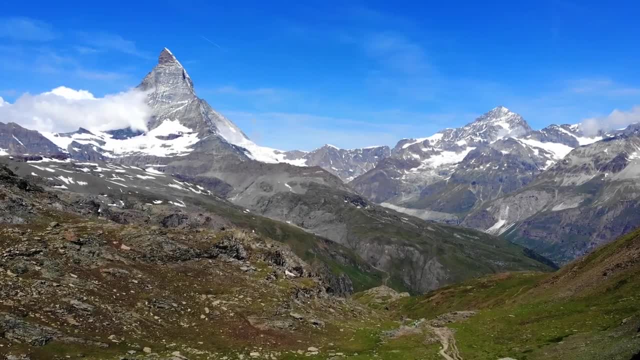 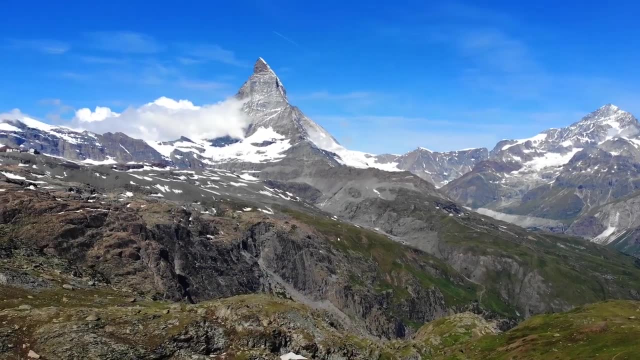 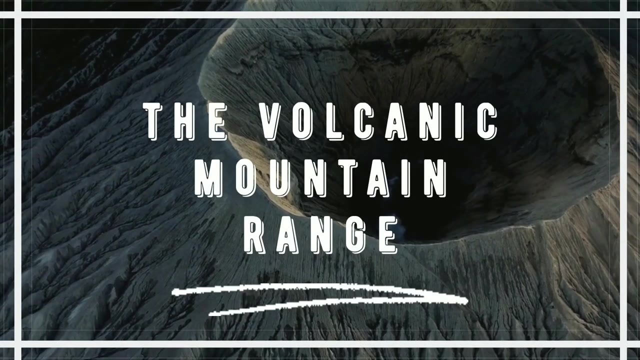 definitively determined. Most agree that it comes from the Cochuca word Ande, which translates to high crest. A minority argue that it comes from Antisui, which is one of the four regions of the Incas who once inhabited the range, The volcanic mountain range, The great majority of the Andean mountain. 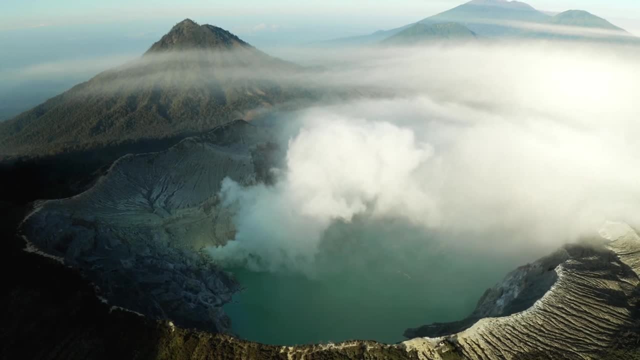 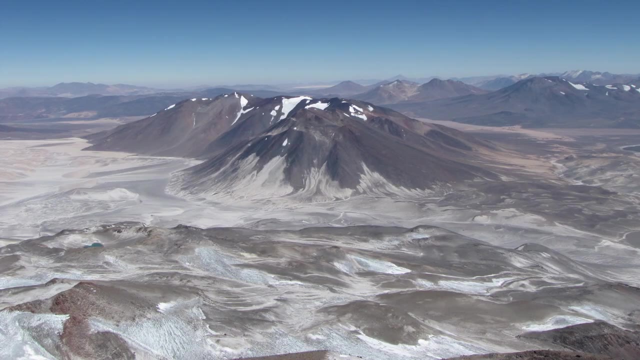 chains are volcanic due to the ongoing tectonic process that formed them. The highest active volcano in the world, which is Del Solado, which stands 6,900 meters, is found here. Parts that are associated with the Ring of Fire, the Pacific volcanic chain, have active volcanoes. 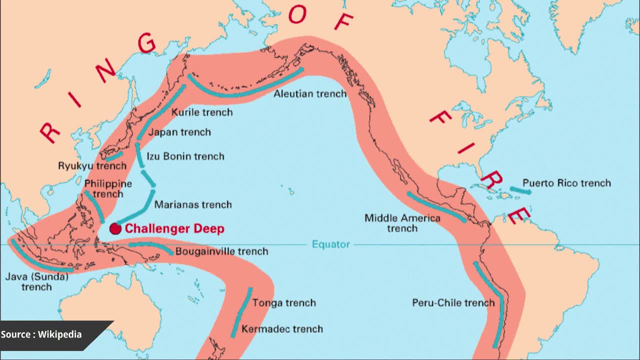 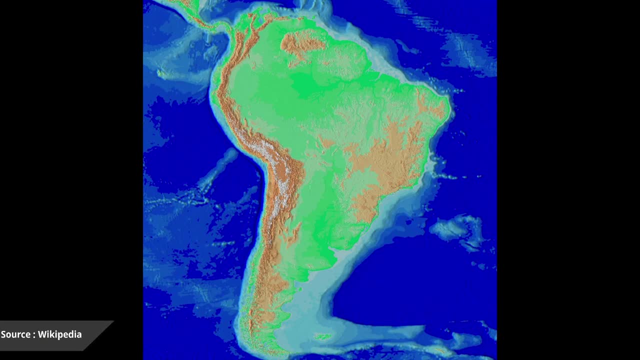 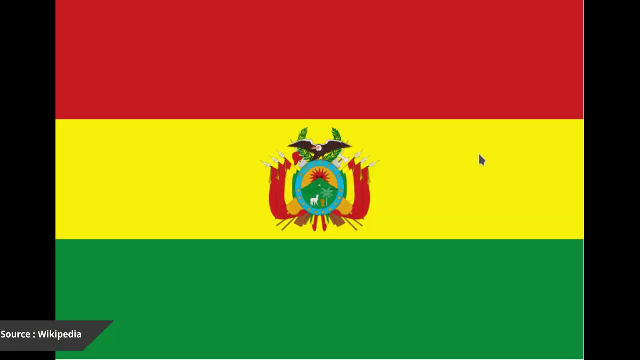 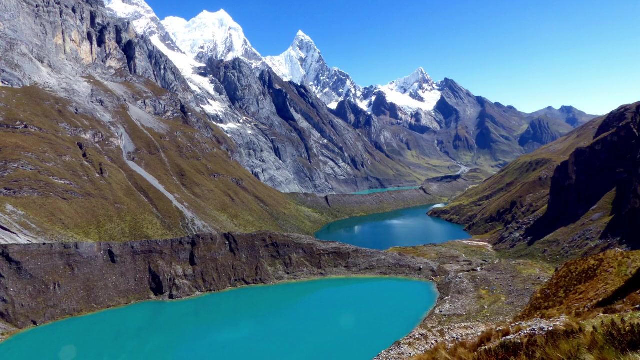 and also, near the Sea, The longest mountain range in the world. The Andes are the longest mountain range in the world. The Andes extended from north to south through seven South American countries- Venezuela, Colombia, Ecuador, Peru, Bolivia, Chile and Argentina. The Andes are the world's highest mountain range outside of Asia, The 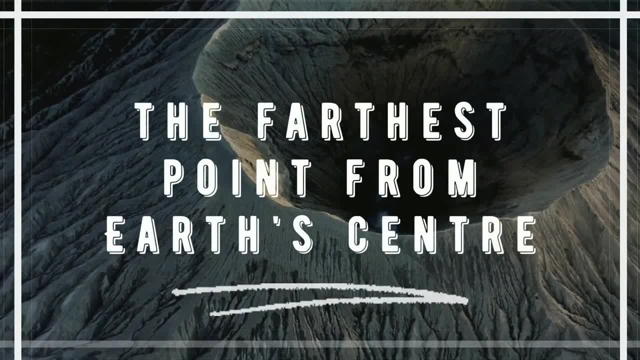 average height of the Andes, that is 4000 metres, is 13,000 feet. The furthest point from our center is the Suez crescent BEA. Crimson waves creep the earth from Olympia and danube tectonics and other rock wollteous rocks that are within rustrom in the state. The most상ed py echtes can be carried out of Asia on beje church of indiana of local temples. 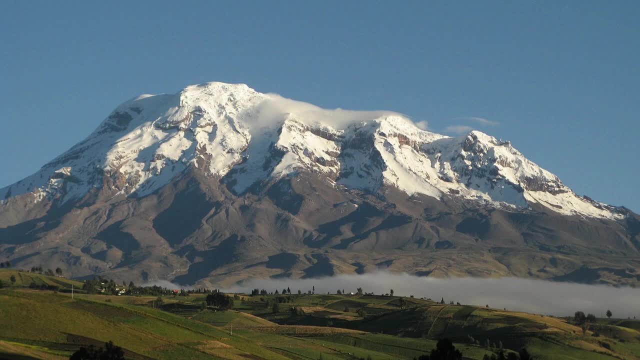 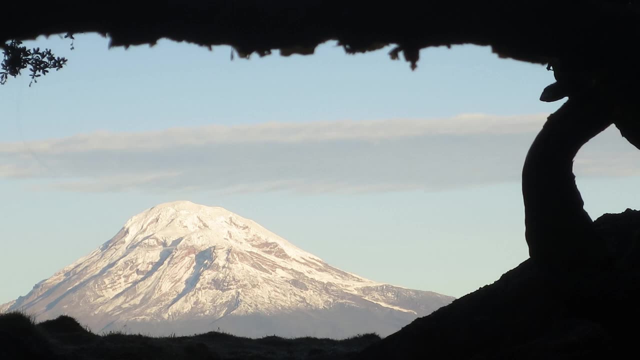 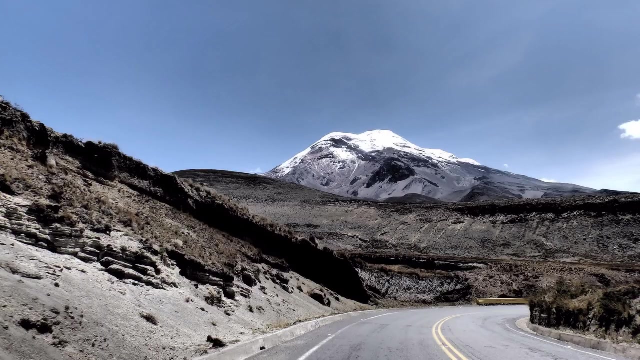 From Earth's Center. The peak of the Cimborazo is the Earth's furthest point. The peak is located in the Ecuadorian Andes, where it rises a height of 6268 m above sea level. The distance from the center of the Earth to the peak is 6384 km, which is 2 km higher. 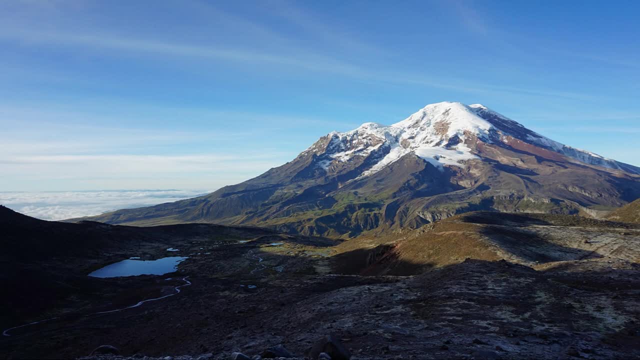 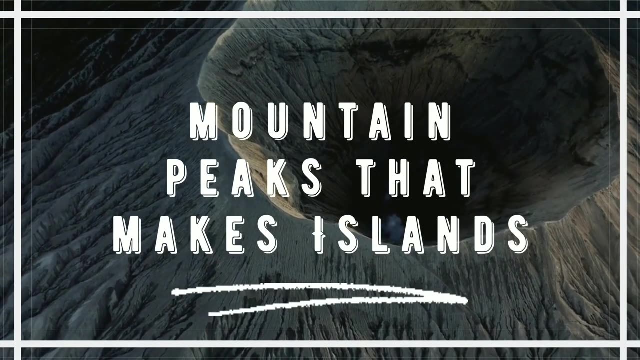 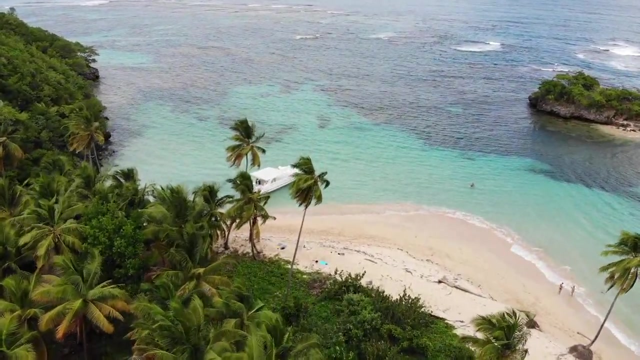 than the Himalayas. This makes the Cimborazo is the only point on the Earth closest to the outer space and the moon. American peaks that make islands Down the southern and the northern tip of the continent, the Andes stumble into the sea, creating a myriad of islands. The Andes are part of the larger American Cordillera, which is a near-continuous chain of mountains which is extended north all the way through North America, the Caribbean, half of Aruba and Bonaire, and in South Patagonia there are numerous islands belonging to the. 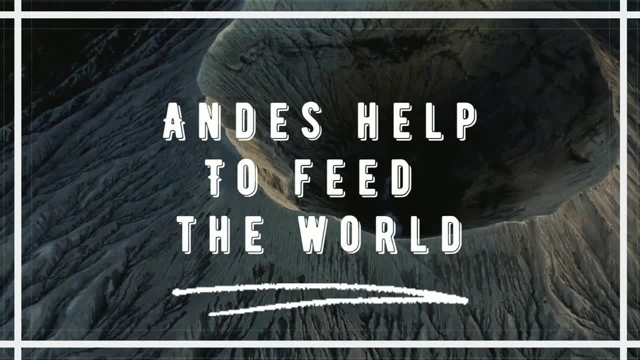 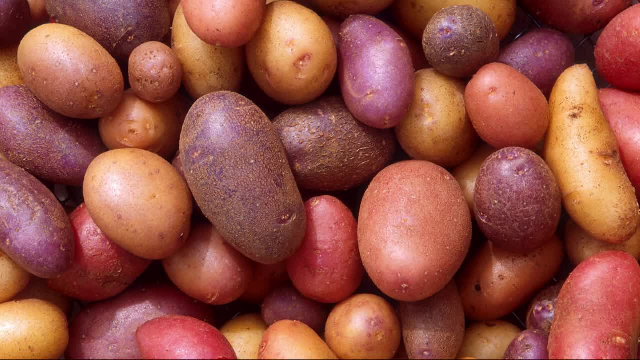 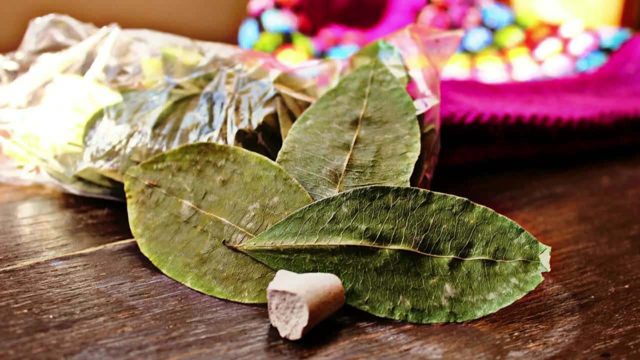 same mountain chain. Andes help to feed the world. Potatoes and tomatoes, two of the most widespread crops on our planet, originate from the Andes. Over 3,800 different types of potatoes are grown in Peru alone. Coca leaves also famously originate from the western slopes of the Andean mountains. 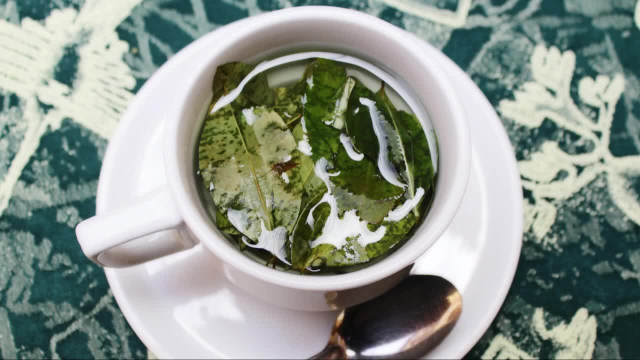 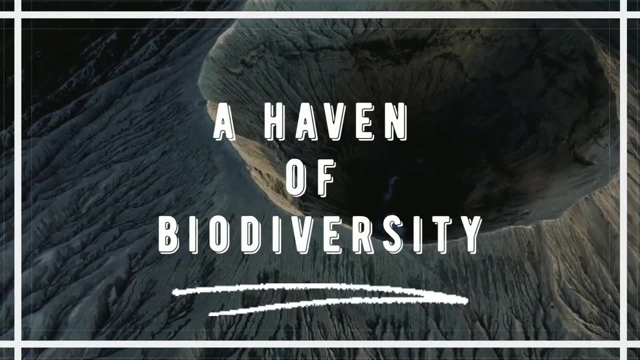 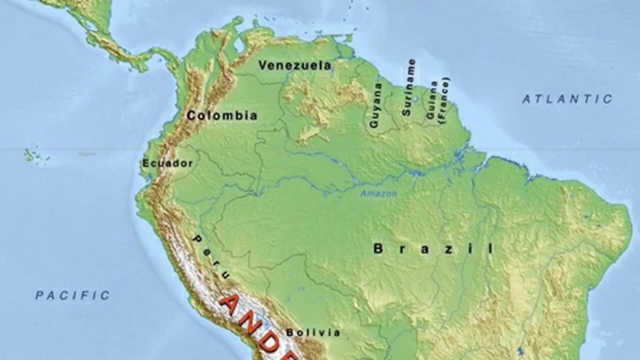 Coca tea is served everywhere in the high Andes and it is one of the effective relievers of the symptoms of altitude sickness. A heaven of biodiversity, The Andes Mountains are known for its incredible biodiversity. They comprise three different main climatic zones, known as Tropical Andes in north Dry. 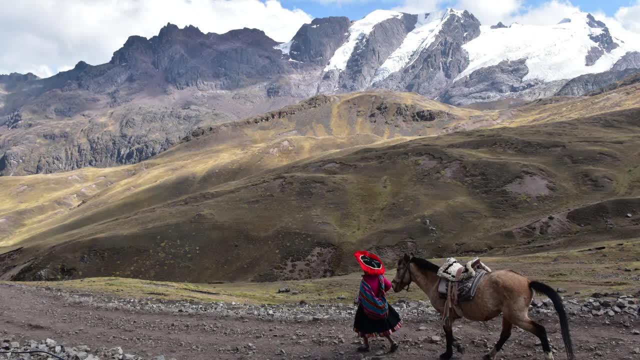 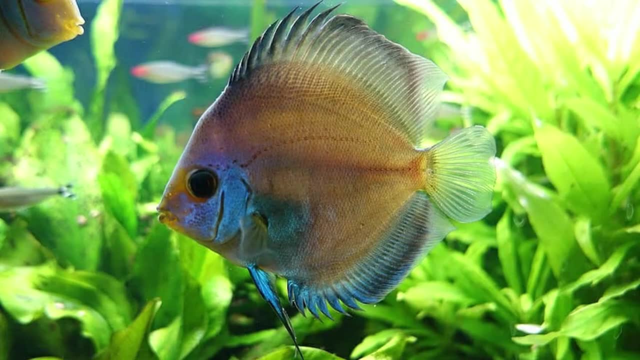 Andes in center and Wet Andes in south. The ranges are home to an astronomical array of wildlife, including just 600 different species of mammals, an equal number of reptile species, 400 species of fish, over 1,700 types. 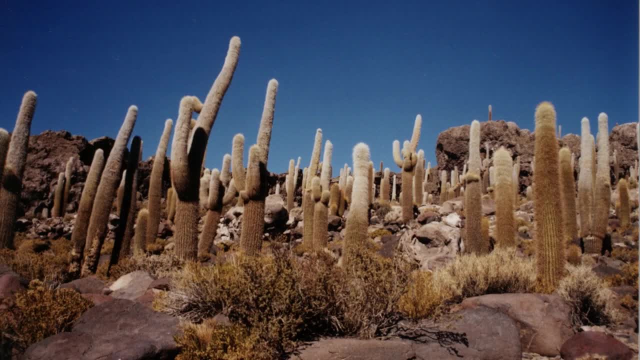 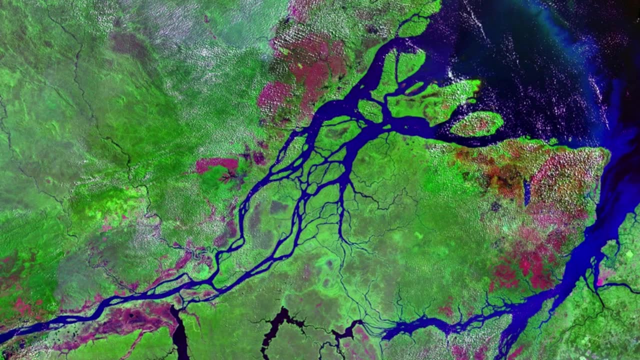 of birds, more than 1,000 amphibians and way over 30,000 species of endemic plants, The Source of the Major River Systems. The Amazon and the Orinoco River systems are the two major river systems in South America. They are originated from the Andes Mountains. 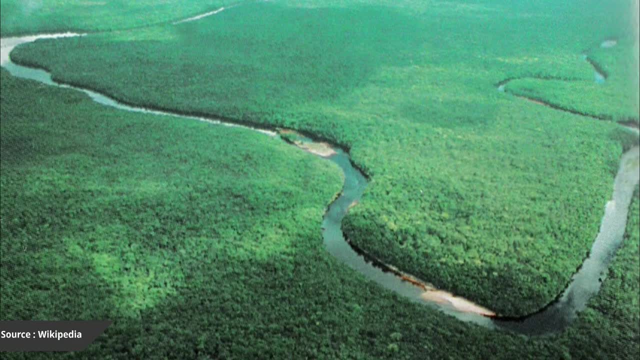 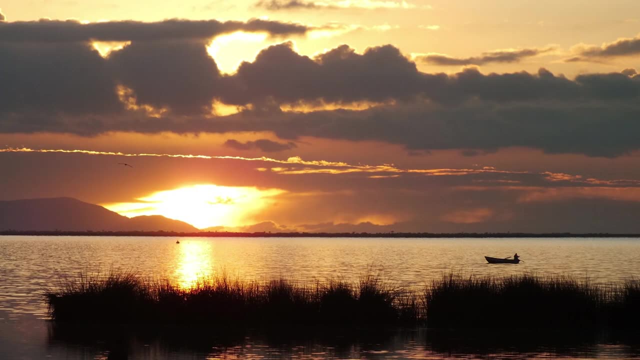 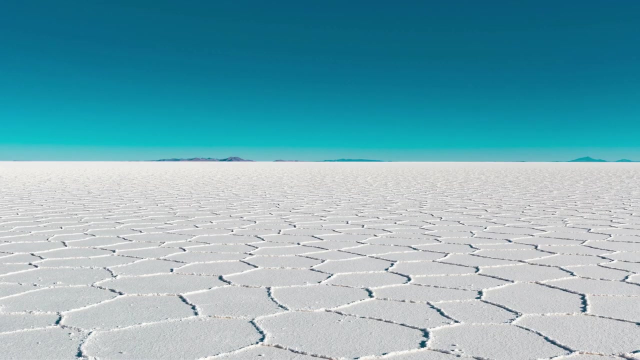 Also, the world's highest water body that can be used for commercial navigation is Lake Titicaca. that is found between the region of Peru and Bolivia. The lake is located at 3,812 meters above sea level. The Largest Salt Flat, Salar de Uyuni, is the largest salt flat in. 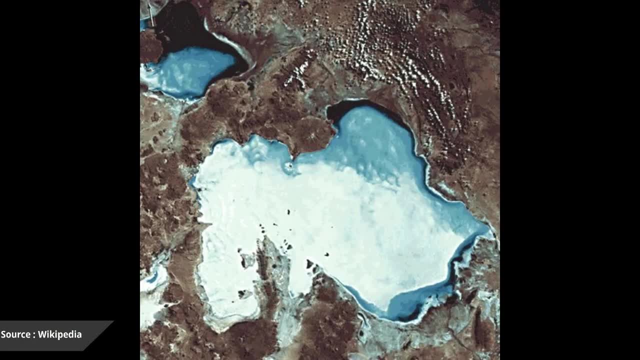 the world that extends for 10,582 square kilometers and is found in the Andes Mountains. in the Andes Mountains, Salar de Uyuni is the largest salt flat in the world. that extends for 10,582 square kilometers. Salar de Uyuni is the largest salt flat in the world that extends for 10,582 square. 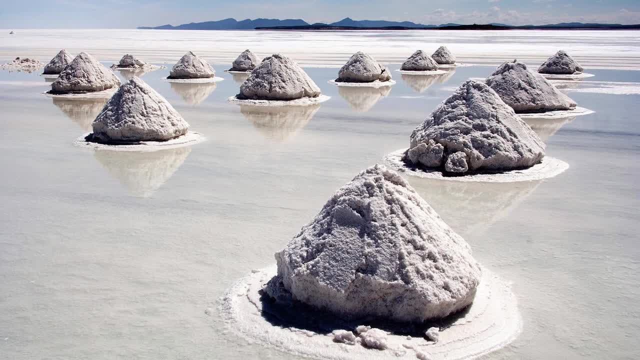 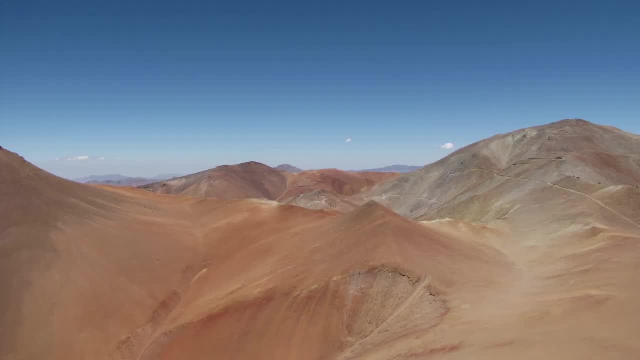 kilometers and is found in the Andes Mountains. in the Andes Mountains, It is located at an altitude of 3,650 meters in the Bolivian Andes, World's Largest Mineral Deposits. The Andes ranges are rich in iron, copper. silver, tin and coal, which have attracted thousands of miners. The largest gold mine in the world is Peru's Llana Cocha, and both Chile and Peru combine to produce almost half of the world's mined copper. Rich in History, The Andes Mountains have been inhabited for centuries. 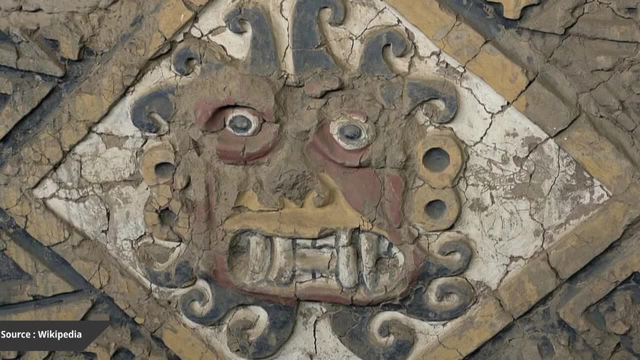 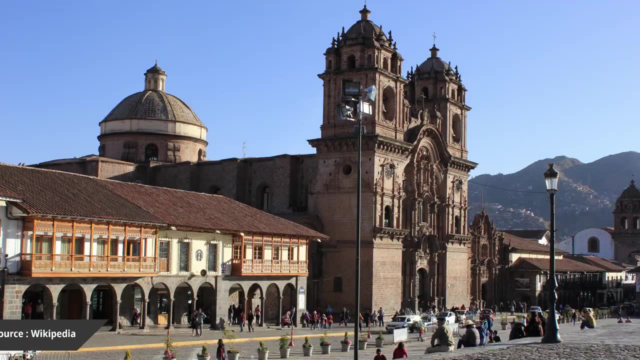 One of the most recognizable civilizations from the past is the ancient Inca Empire. The Inca engineers built massive, impressive sites, including Machu Picchu and the capital city of Cusco. The Inca also constructed roads and conduits throughout the mountain. 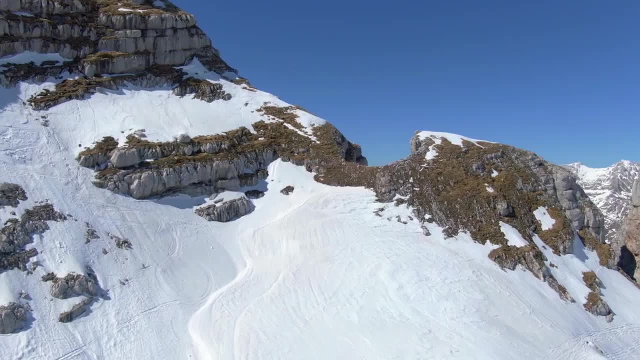 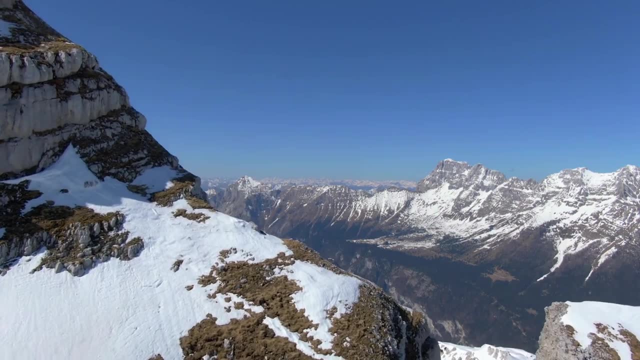 The True Highest Point on the Earth is Right Here. Due to the equatorial bulge of our planet, the peak of Ecuador's Mount Chimborazo is actually the furthest point from the Earth's surface to its core, At 6,263 meters. this is Ecuador's highest peak and is considered inactive due to the